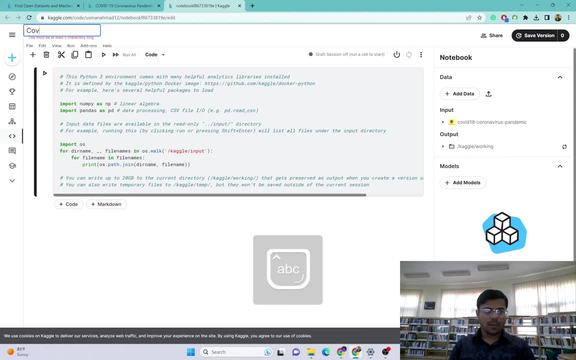 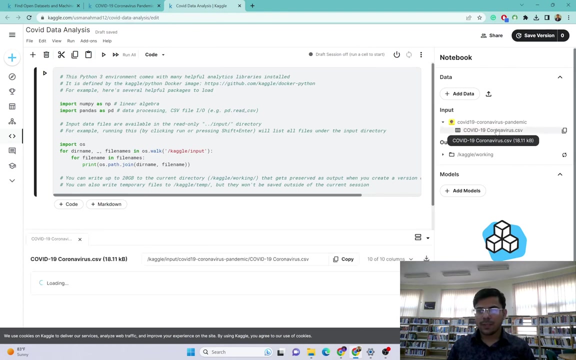 covet 19 data analysis. and okay, so the title forever 19, data analysis already exists. so, uh, i will just write it: covet data analysis. okay, it's, it's fine now and once we uh create this new tab here, create this new notebook here, you can see the data set is already there as input and you can see this is the file. 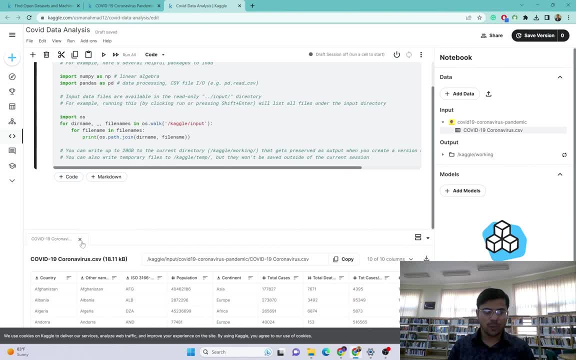 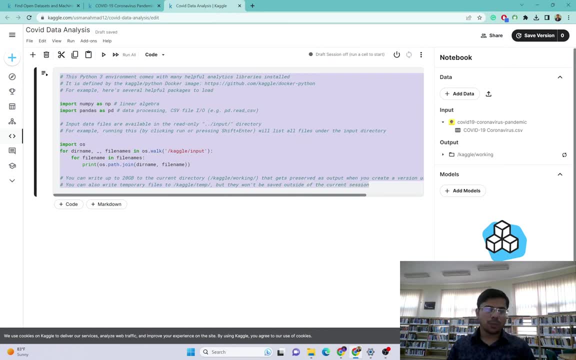 and you can access it this file here. this is the preview of the file and you can see Kaggle will automatically import some important libraries. so import numpy as np. this is for linear algebra and for data processing. we have csv file here, so definitely we will be needing pandas library. 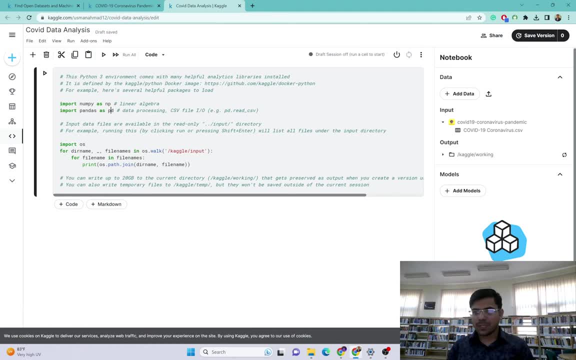 that will be specifically working on csv files, and then we, the Kaggle has already loaded or linked the data set with this new notebook. so at what I will do here, I will just run this statement, run this line of code, and once I will get any output here, it means: 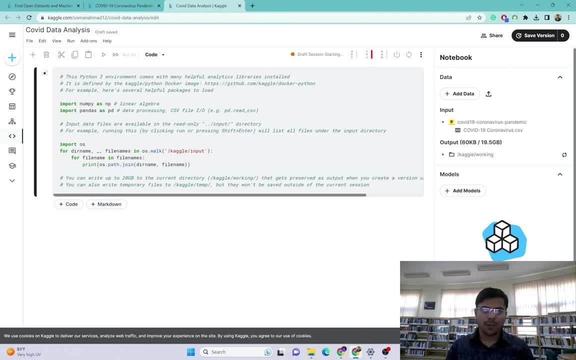 that our data set is properly linked with the new notebook. okay, so just wait for the instruction and you can see these online resources are being used. so you can see cpu ram, and ram is maximum 30 gb- that is massive. and disk and we have session, so disk space is also also available here. so now this is live, so you can see the. 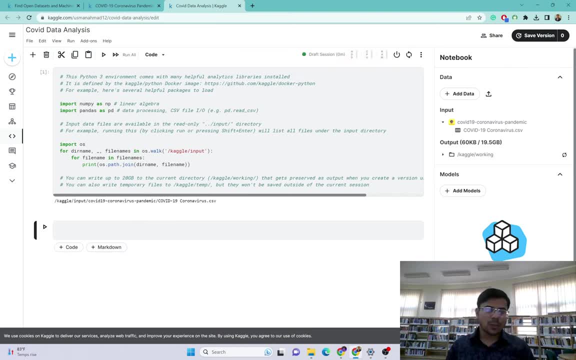 green means that this is running. I will create a new code here, so I want to explore this data set. so what I will do? data- okay, let me just create a page. so this canvas. I will create thiseger saved it okay, so I'm gonna save this my record, and I'm standing here trying to create this. 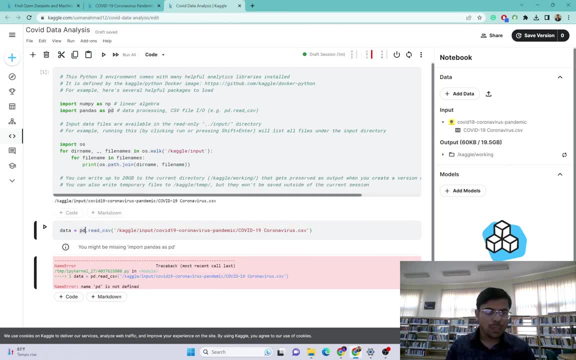 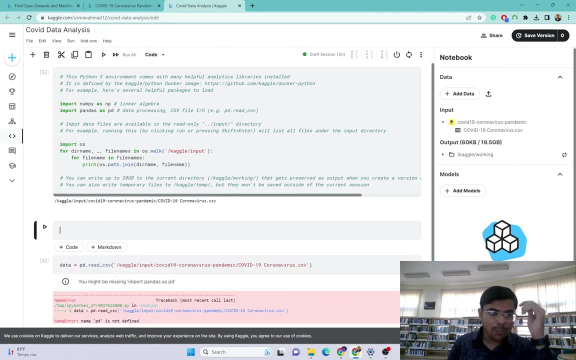 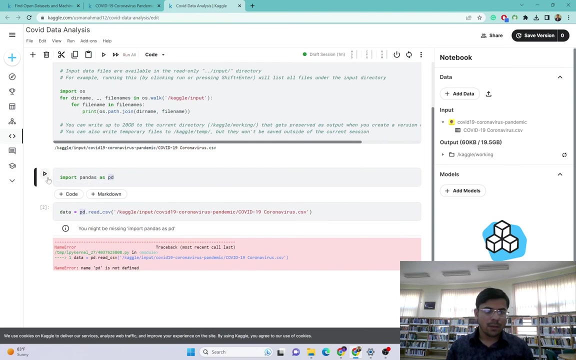 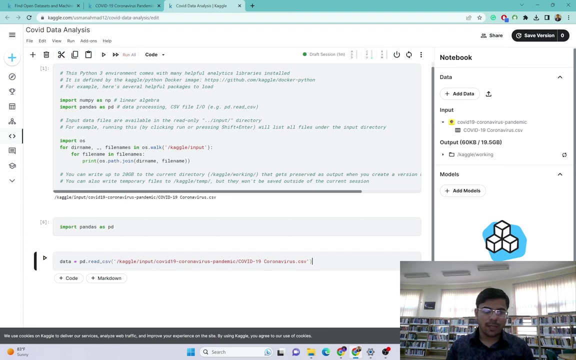 area I have. my standing exists in my library. okay, this is ok. so this is already imported, but let's import this again. import pandas as pd. run this, ok, and now let's rerun this. and now it is not giving me any error. it means that our 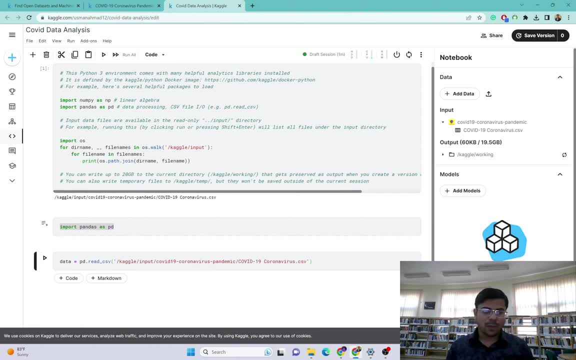 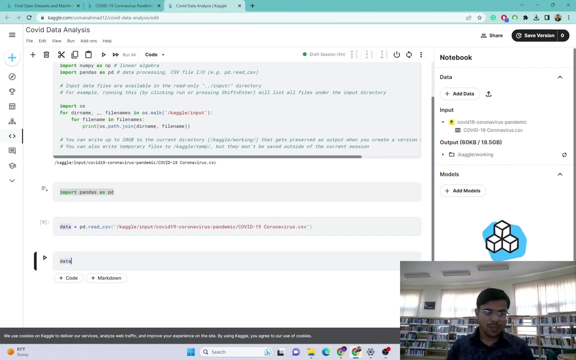 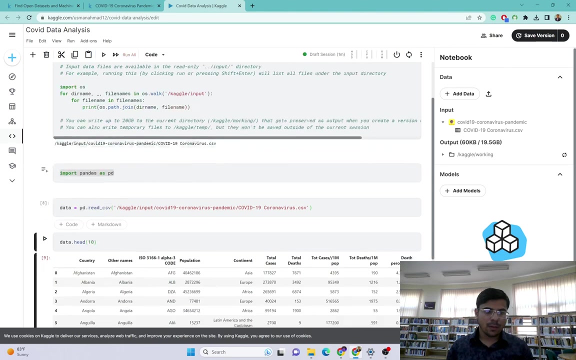 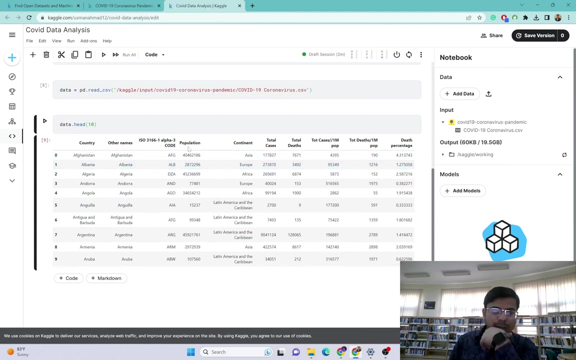 pandas library is fine. so now I will explore some values in this data set. so I will write datahead and I want to print first 10 values in this so you can see in this data set we have these columns: country, other names, population, total cases, total deaths and all these data values are 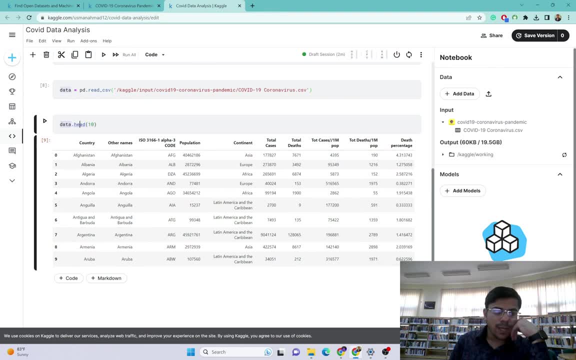 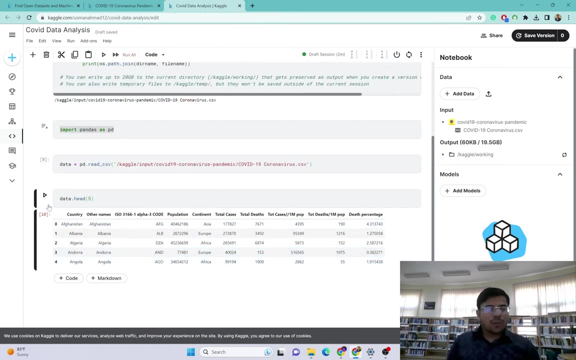 available here, but you can see the head will be giving you the first, whatever the first values, number of values we need. so, for example, if I write 5 here, so it will give me 5 values right now. I want to see what this data is about. 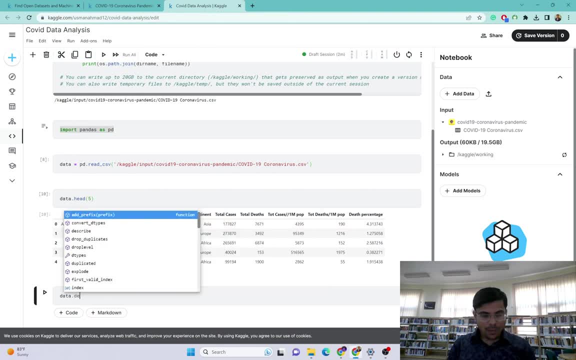 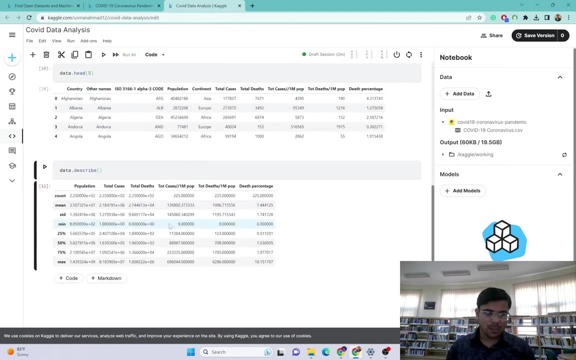 so datahead, and I want to describe function. let's see what this data is about. so these are the total values and mean value. this is very good for data analysis. 25% values, 75% and this is the max values, ok, in each column. so this is very effective and I want to see how many rows. 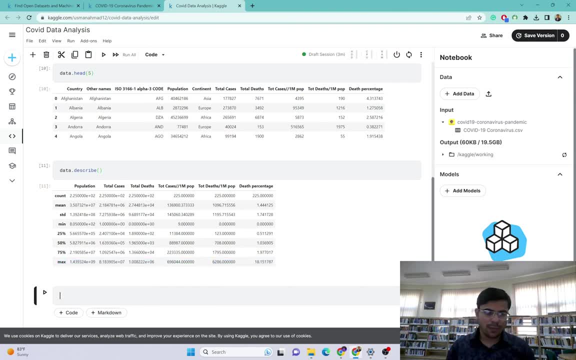 and how many columns are there. so for that we have another function here, and this is the Boolean function, and so let's run this row here to describe which values does that form. so now again we have. so this is the main function, that is, datahead function. we. 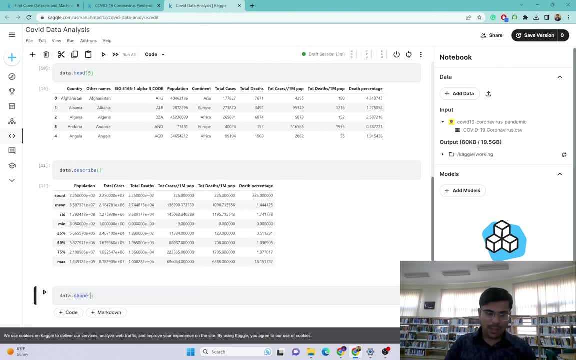 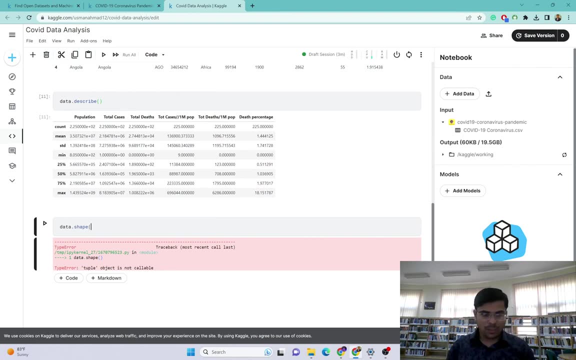 have to dear who are the main function, that is datathe shape function and that's round this. okay, so datash está 820 туда a, pero no tenemos qué tal plus. no sabemos nía na. hence vamos a los compositions royalty. so our purchasesanti haberacji. 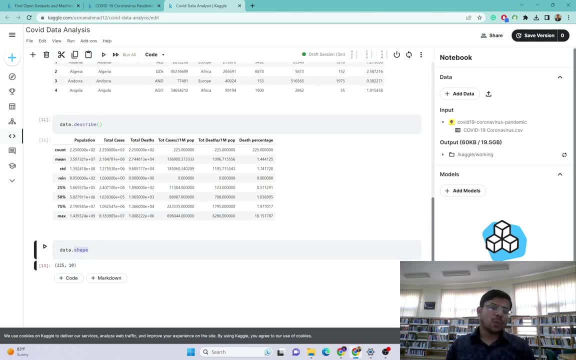 okay, so in the example how we have 225, but we also exceptos 3, we have skinpear the number. this is the shape of this data: we have 580 dalas. so their license, the production, to see if we want to see this column down below a bit. 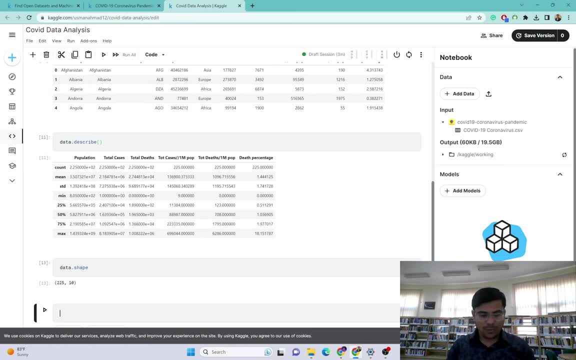 lower. and then we have, we have, we have the Furly minister ing 10, we have, or left, and this is a 25, that's the a audio relative network status. so let's hit that, that and a whole. you have to go to a the last values. so that will be data dot tail. this function will give me last five values, i think. 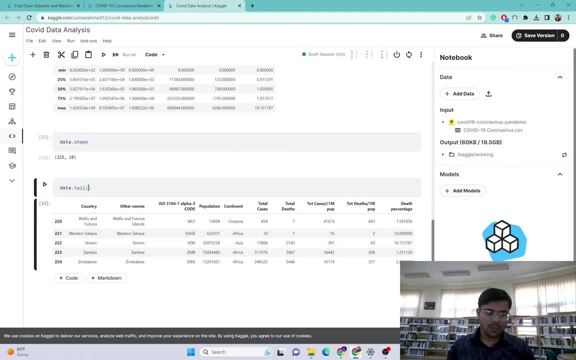 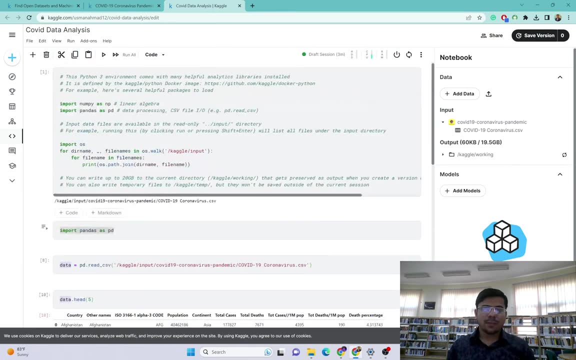 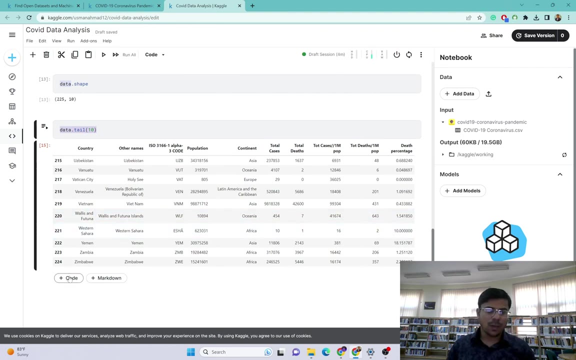 so you can see this is giving me last five values. so if i want last 10 values, so you have to type according to that. so you can see this is pretty much simple and you can, you know, save this and whenever you want to resume the work, you can just resume it from the point you have left. so for 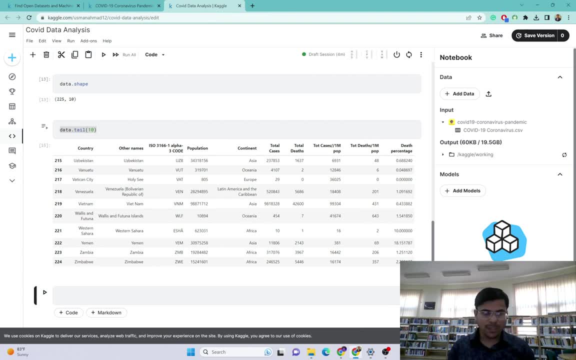 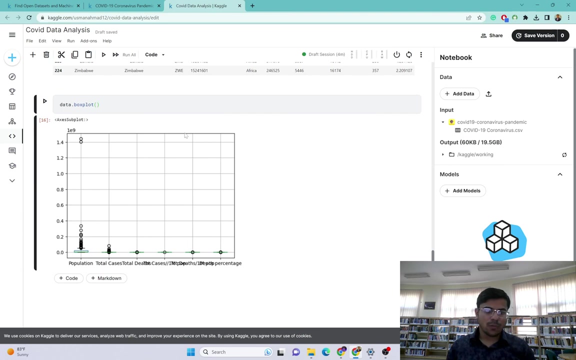 example, i want to plot some graphs. so, for example, data dot box plot. let's see if this one is working like this. okay, so you can see, this is a box plot for this data set and you can explore this one. similarly, we can create histogram: data dot. 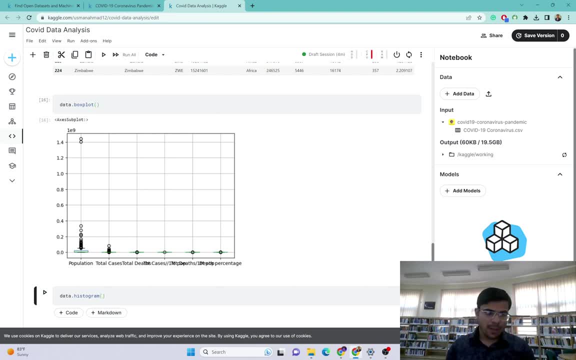 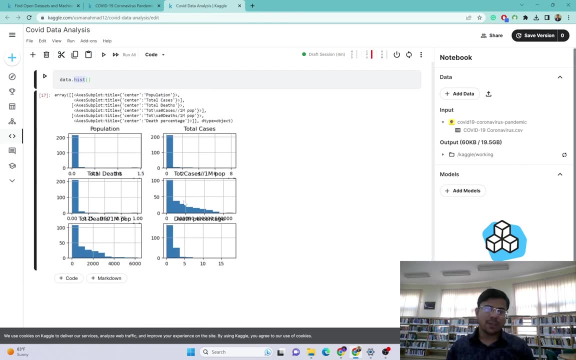 histogram and no, this will be only this. i think yeah, so you can see, this is creating the histogram of the data set. so this one is very effective like this is very effective method. so once you complete this analysis- this is just a very simple way to do it, so you can see that this is a box plot for this data set and you 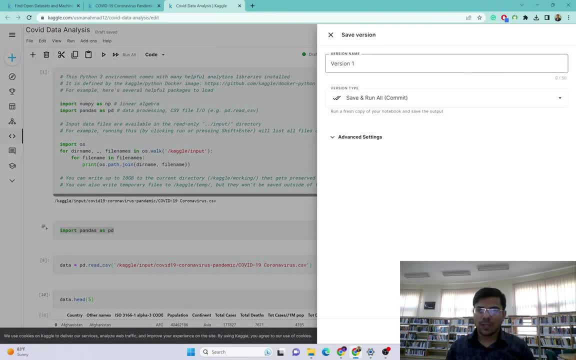 you can see this is a box plot for this data set and you, the example, go to this save version option. save this is so you can write the version one. this is v1 save and you can go to advanced settings and click on save. so this is saving. 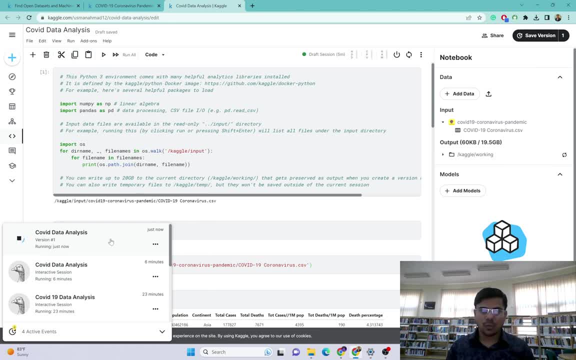 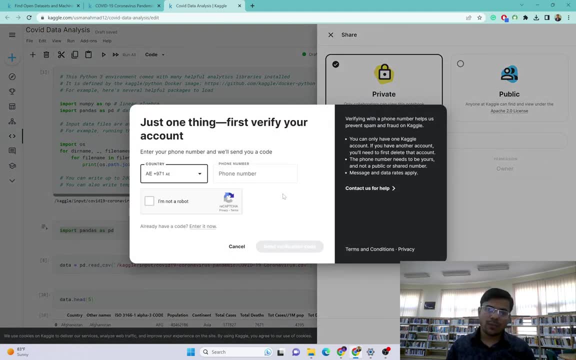 now you can resume working on this project anytime you want, and if you want to share this, what you have to do? you have to click on public, and here you need to verify your mobile number so that then, if you want to share this structure. this is all worked out, and now let's move on to the next one. 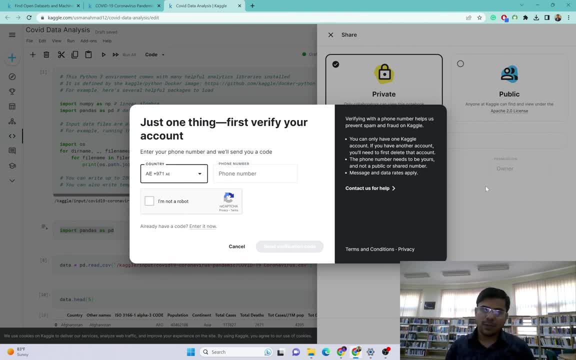 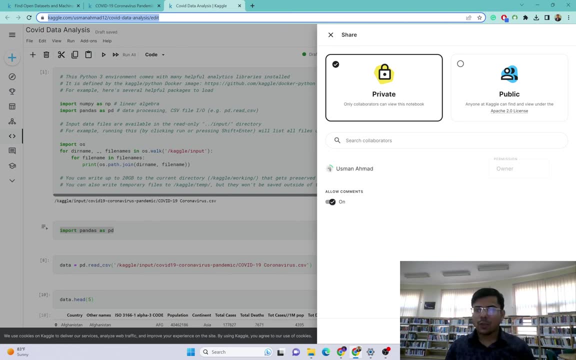 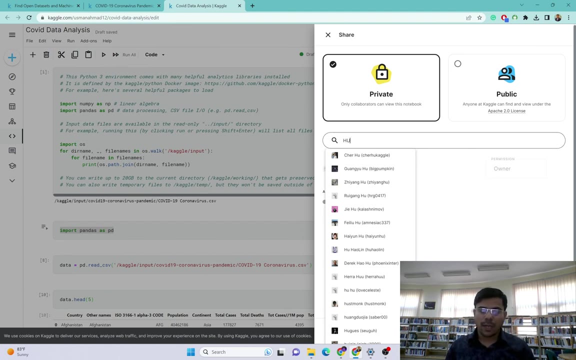 it will be public and it will be easily available for anyone. then you just need to go to the link of this and copy the link and share with any anyone you want to share, so you can also share with any you know online user or any user who is registered with this gaggle. so this is very effective.